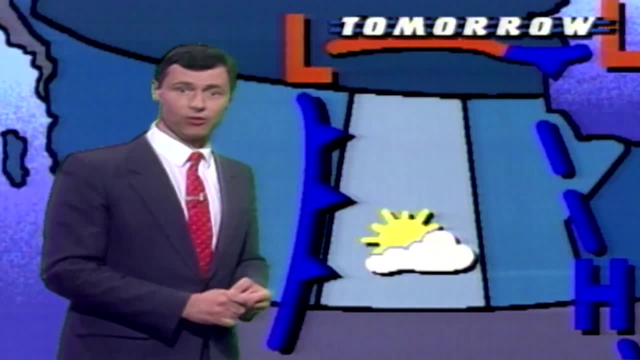 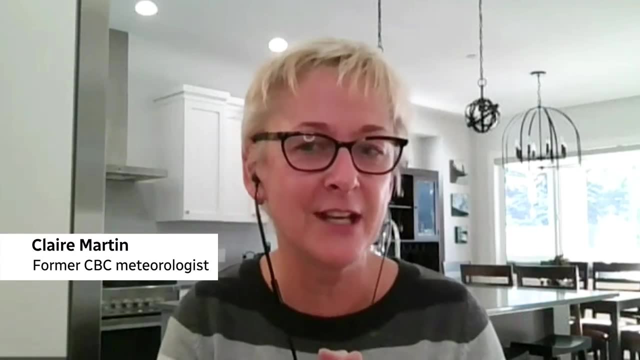 but then technology really started to change in a hurry in the 1980s And former CBC meteorologist Clare Martin started just in time to see it firsthand. We used to get forecast model data on what was called mold facts. It was huge sheets of paper. 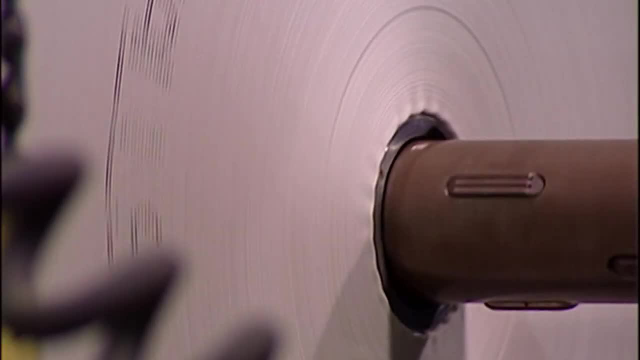 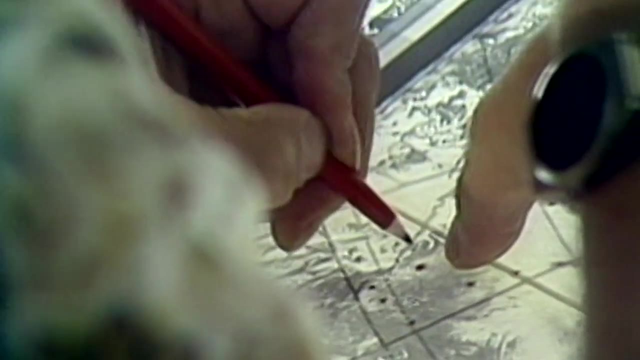 that were wet because they'd been printed like an old newspaper printing press, Highly flammable, probably not very good for your health, And we would draw maps on that. The gentleman that worked performing had still a marker, a pen and a big, huge map. 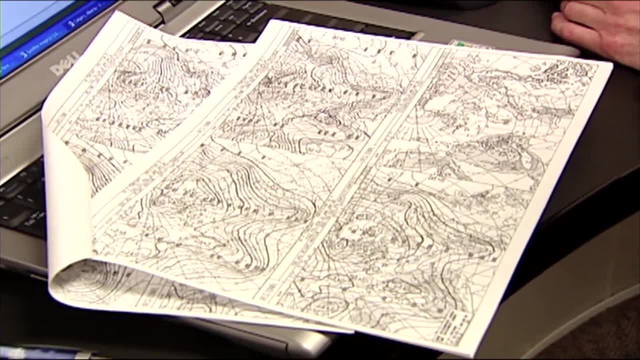 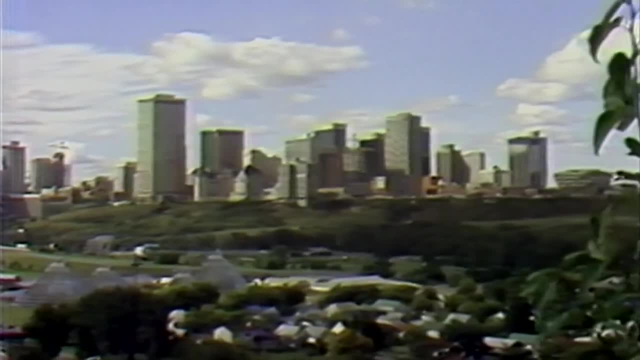 I was slightly more sort of advanced technologically speaking And we had automatic weather stations put around Edmonton which was just massive. I could tell that the temperature in Sherwood Park was different from St Albert, which was huge. In the 90s, computerized graphics made their way to the forefront. 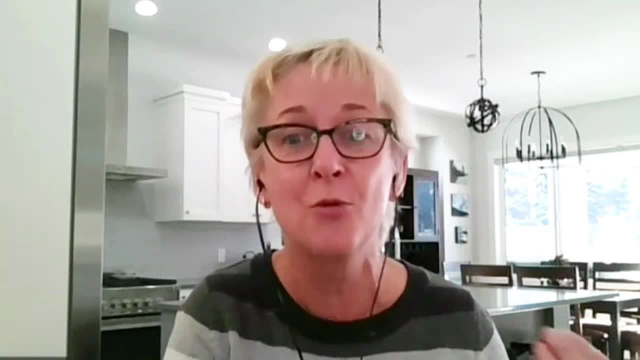 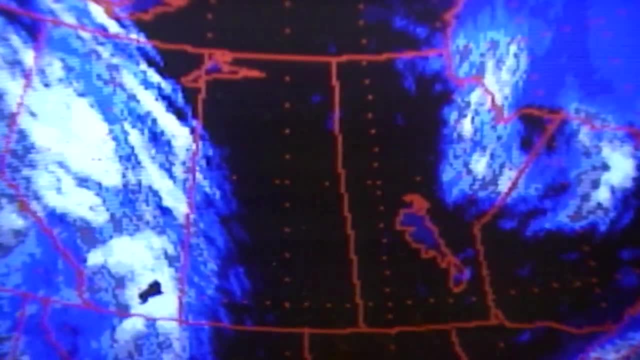 It's akin to having a black and white TV with like four channels- which I grew up with my friend- to satellite TV: all the colors, pick and choose, streaming when you want it, With computer models and graphics. we could see weather, as it happened. 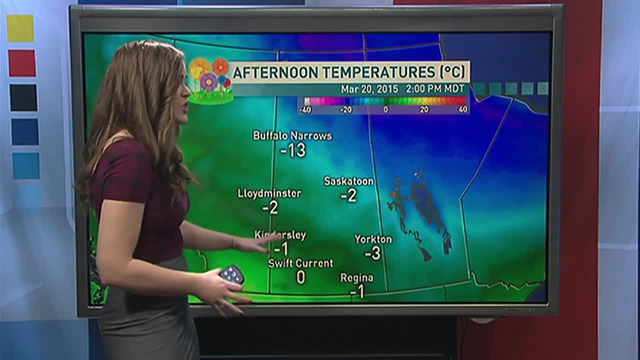 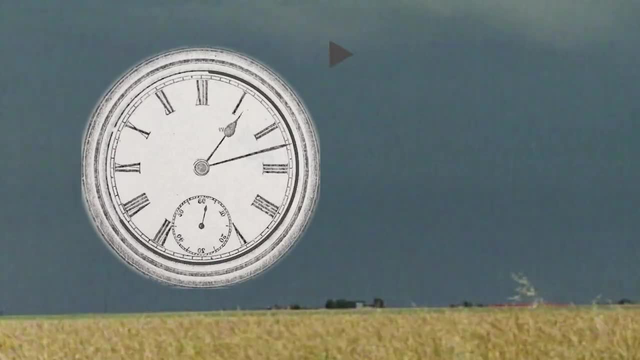 visualize low pressure systems, see the downdrafts for thunderstorms and where hail was forming, And, of course, more information also makes for a more accurate forecast, especially when it comes to the next 24 hours. I've already used TV graphics that are a 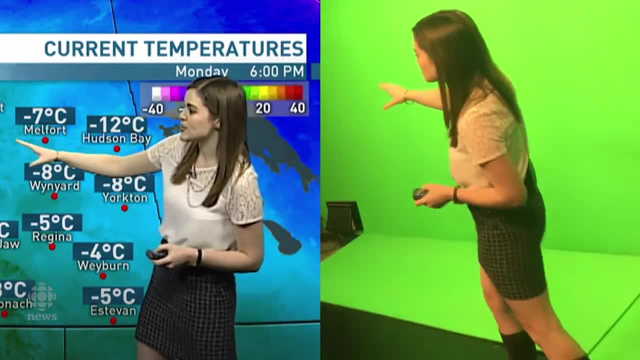 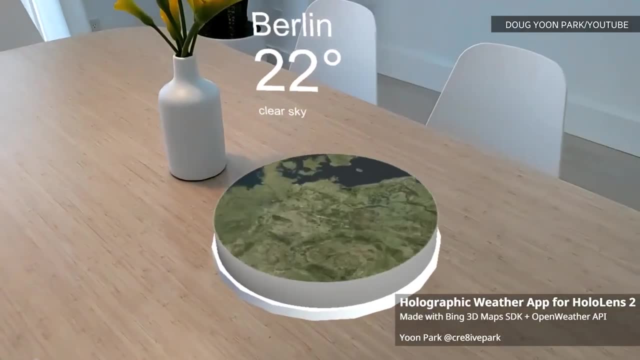 little more modern, like these for 10 years. but where will weather reporting go next? We've already got holograms, virtual reality and interactive 3D green screens, so the sky really is the limit, And that makes some of the veterans a little jealous. 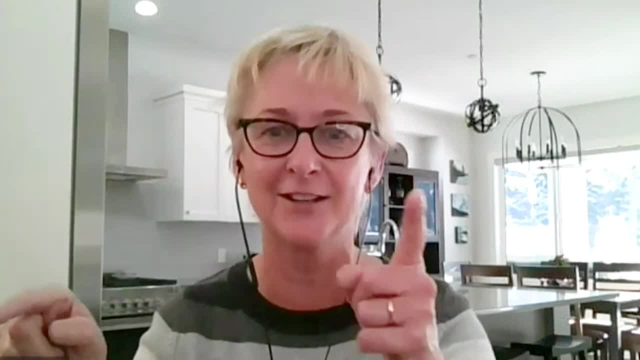 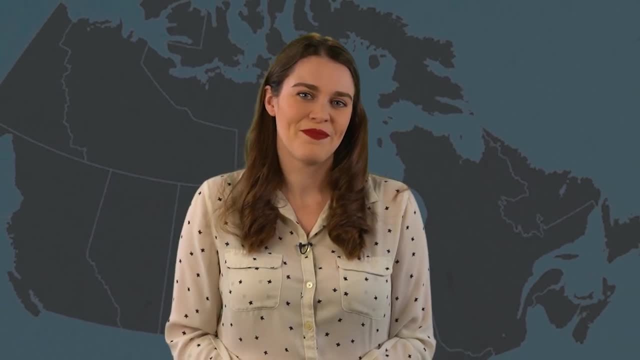 I'd like to be around today. If I get a second chance at a second life, I'd love to do that. And hey, it sure beats delivering weather by Morse code. Christy Klyman-Hagas. CBC News- Edmonton.